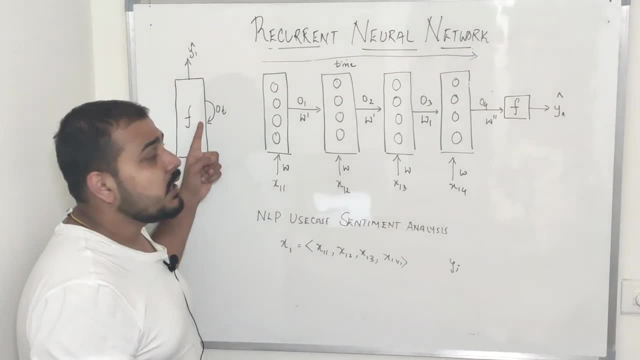 one word. The pre-processing will happen over here and then it will give you an output, and apart from that, for the next word, Whatever was the output for the first word, that will also be sent to this particular neuron and recurrent neural network And because of this, the sequence information is kept. OK, Now I'll. 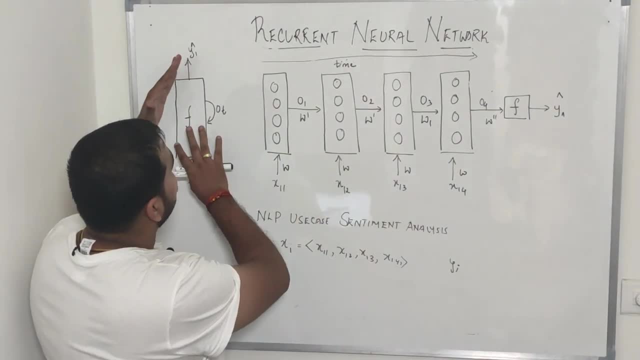 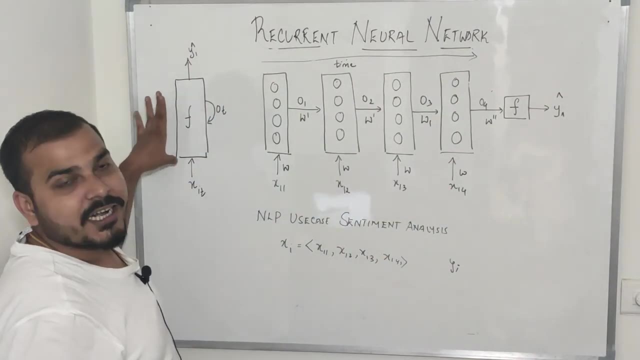 make you understand what exactly I'm telling you, I'll try to expand this whole diagram over here. OK, This is how my whole diagram will look like Now. see this: This is my general architecture of a recurrent neural network. So I told you that I'm trying to solve this NLP use case sentiment. 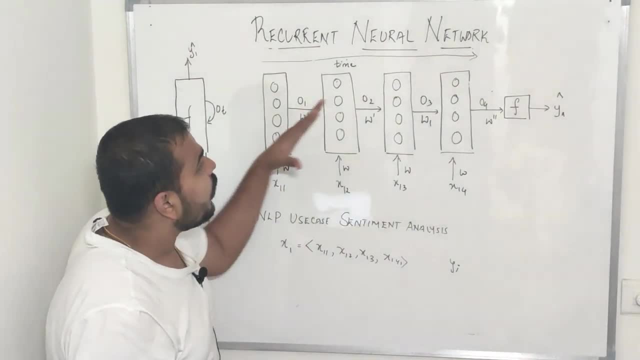 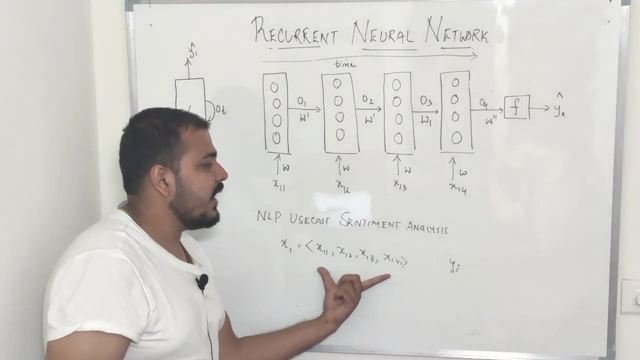 analysis, And I'm discussing about the forward propagation, How forward propagation will take place. OK, So let us go ahead and try to understand Now. suppose I have these four words. OK, And this is my output Now. at time t is equal. 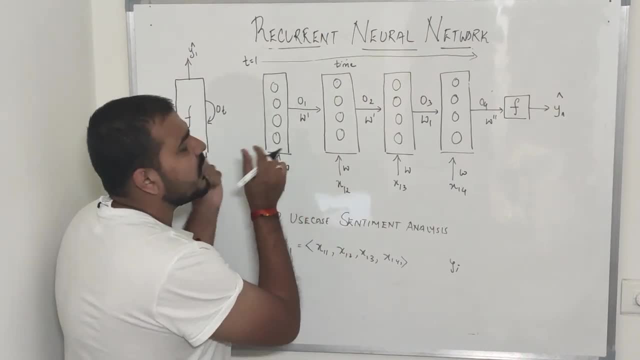 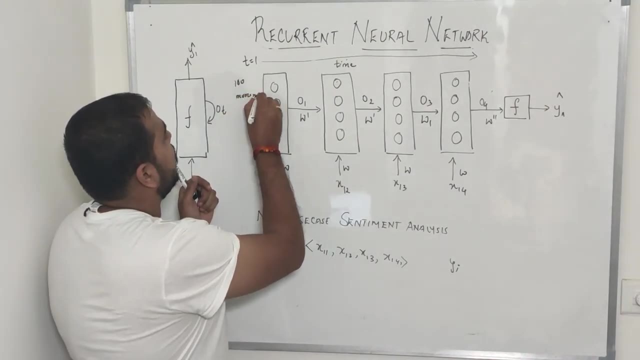 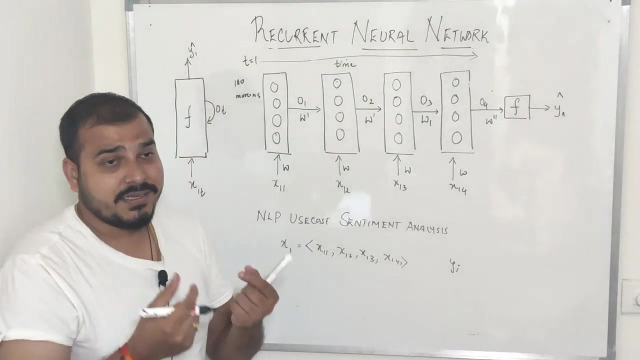 to one. My first word goes: inside this particular hidden layer. Now suppose, in this particular hidden layer, I have 100 neurons. OK, I have 100 neurons. Now what will happen? The first thing that will happen is that this input, this word, and I can represent this word. 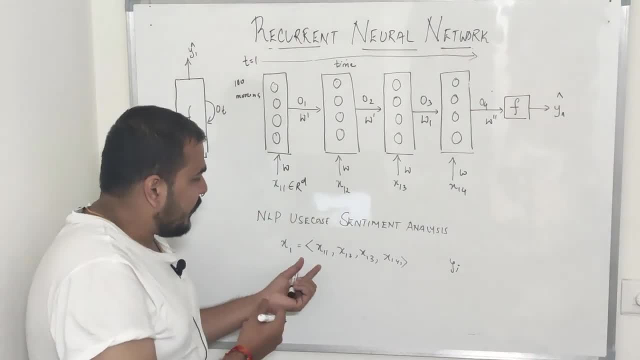 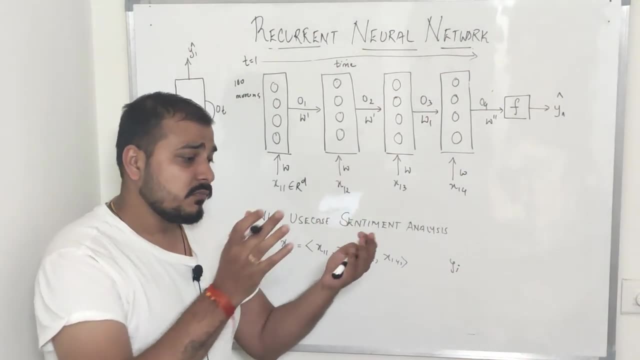 Into some dimensions, that is, of RD. So I can represents this with some vector. You know this word: I can represent with some vector And how to do that. I'll show you that in the practical application. And if you know about word to work here, if I do, you have a bag of words. 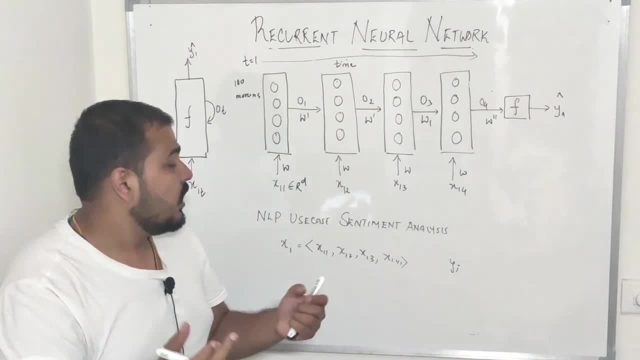 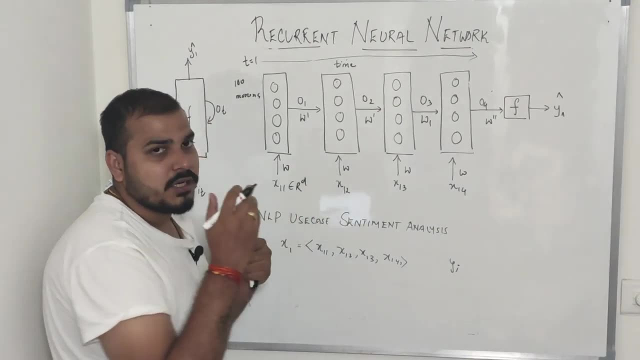 there, each and every word, we try to represent it in the form of vectors, right? So, similarly, this particular word will be represented for some d dimension vector. Then we assign weights, because this is how in ANN also happens, Right, We have our input, then we 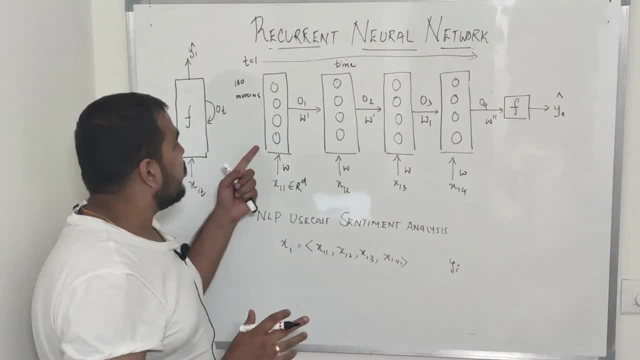 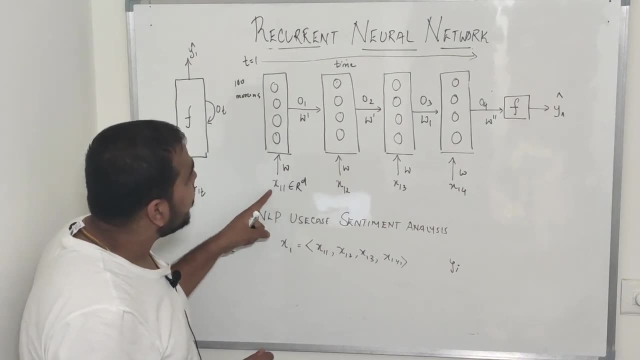 multiplied the weights and then we give it to the hidden layer. so this hidden layer is having 100 neurons, right? so suppose this is having 100 neurons. so i will try to multiply my input layer, that is, whatever the input data, i'm coming along with this particular weights and i'll get the output o1. 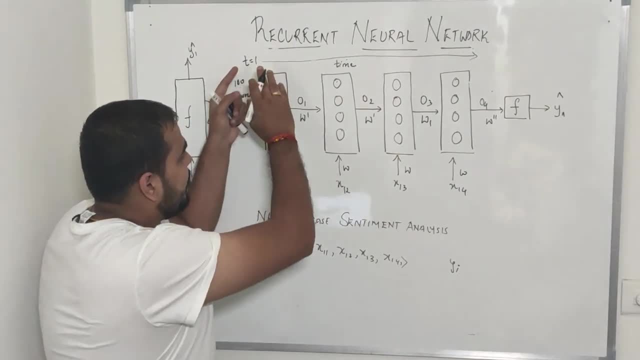 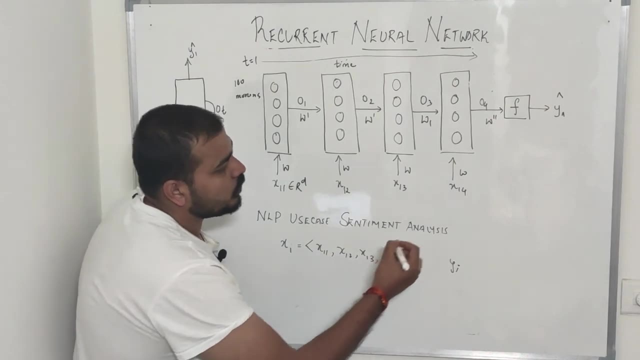 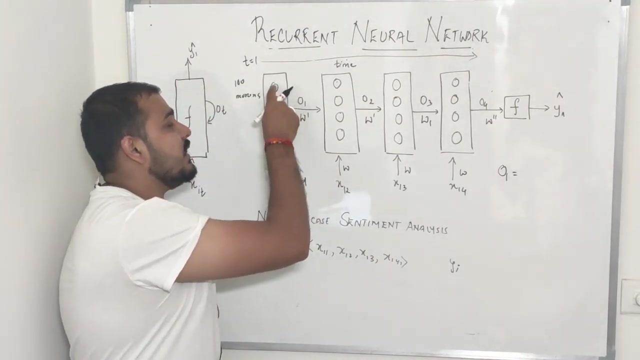 okay, now, this is at time is equal to one, at time is equal to one. i'm just passing one input right now. okay, so let us go ahead and write the first function of o1, so o1 can be written over here as okay. so here i'm actually now and understand one more thing, guys, here is all my hidden neurons. 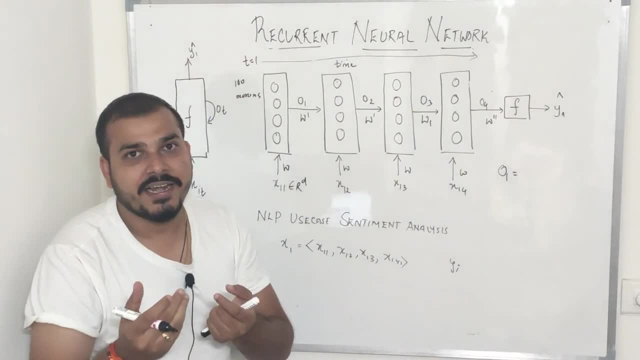 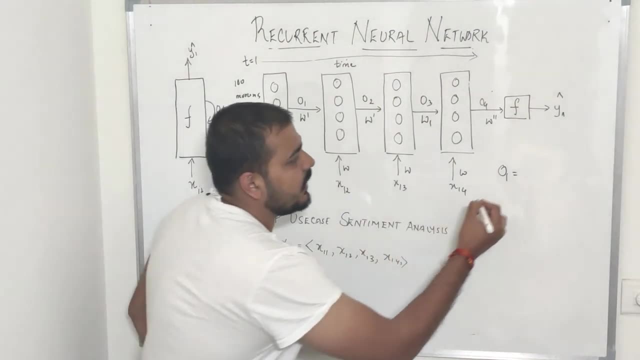 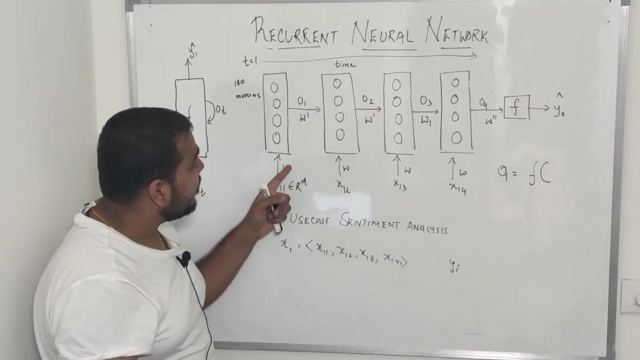 and you know that in hidden neurons i apply some activation function right, like relu, like tan h, like sigmoid activation functions. so this o1 will basically be some function. right, i'll apply some kind of function over here and in this function we'll try to multiply w and x11. that is what we. 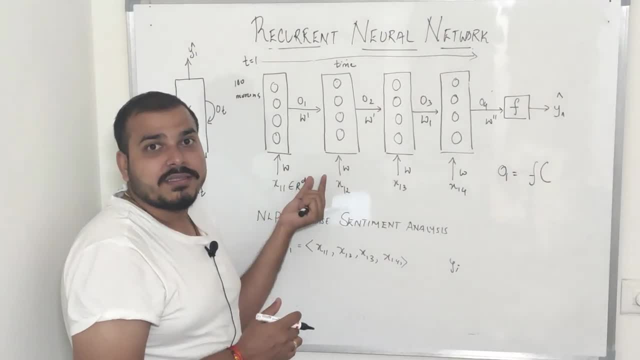 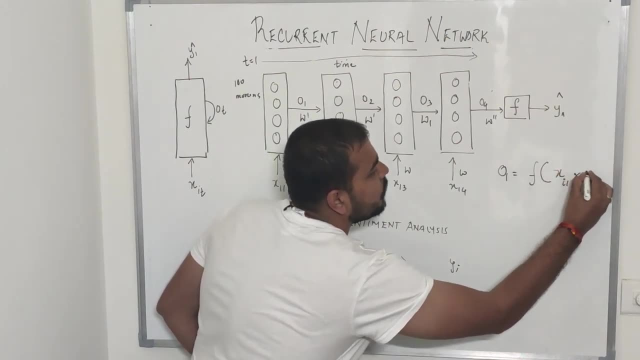 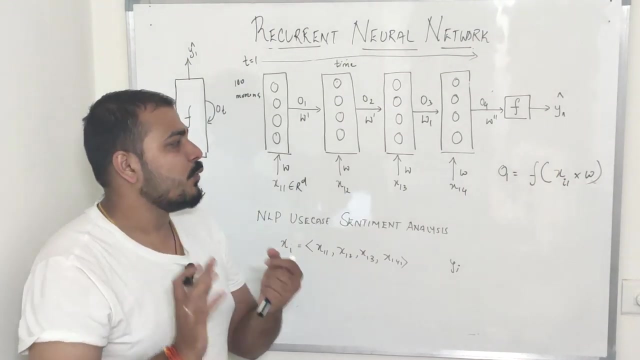 do right. in ann we'll multiply the inputs along with the weights in each and every hidden neuron. so here i can basically write it as x, i1 multiplied by w. okay, so this will be my output one. okay, this will be my output one. pretty much clear. okay. 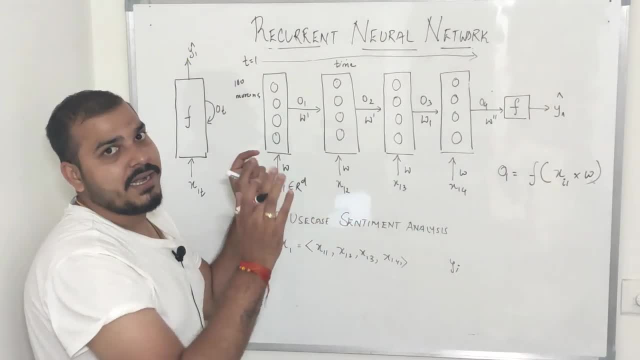 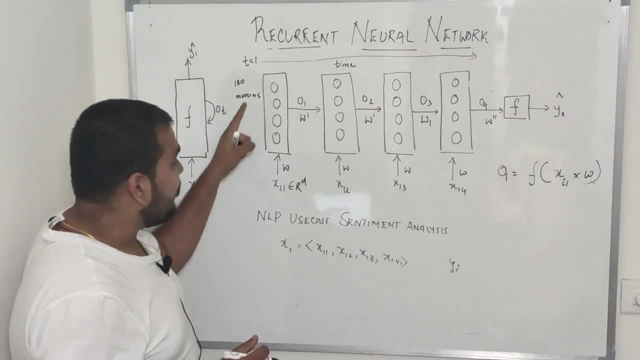 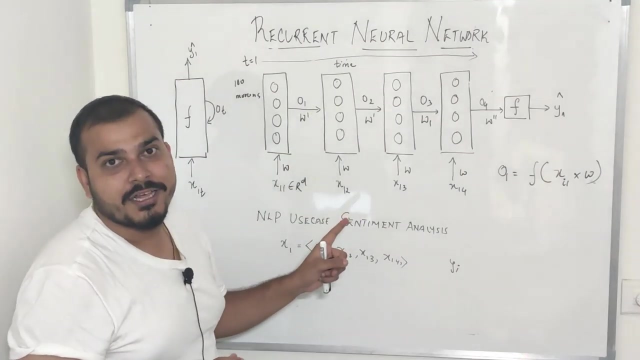 and this is important. this is what is happening in the forward propagation right now. once this output one is computed, now again go back to this architecture. now this output one has to be given to the same hidden neuron, right? so this hidden neuron again will come over, okay, and same number of hundred hundred hidden neurons will be coming. but at time is equal to t. 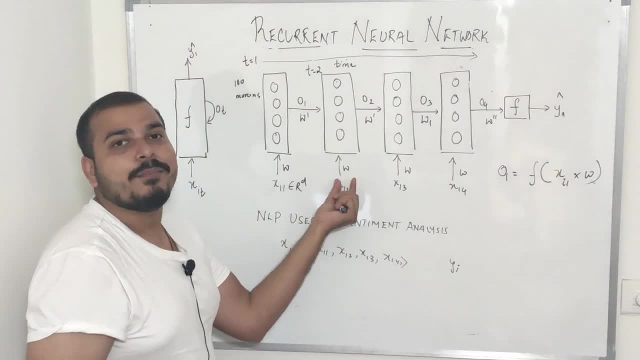 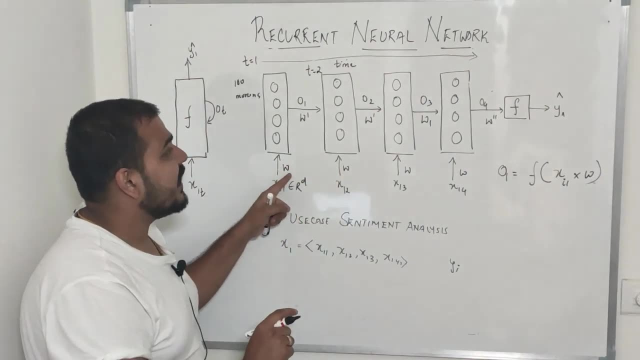 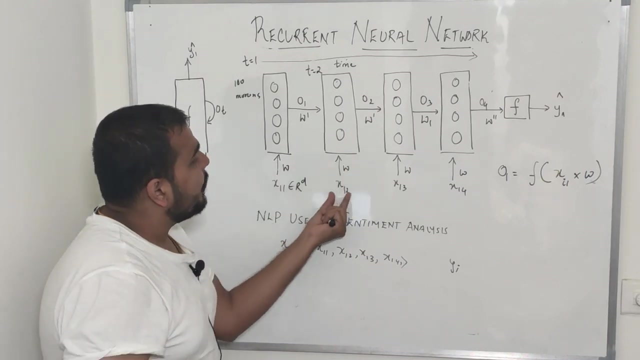 is equal to 2. my next word, that is x12, will get passed now when it is getting past. the same weights will get assigned over here. remember guys, weights will get updated only in the back propagation, not in the forward propagation. so in my t is equal to 2, the same weights will get assigned. 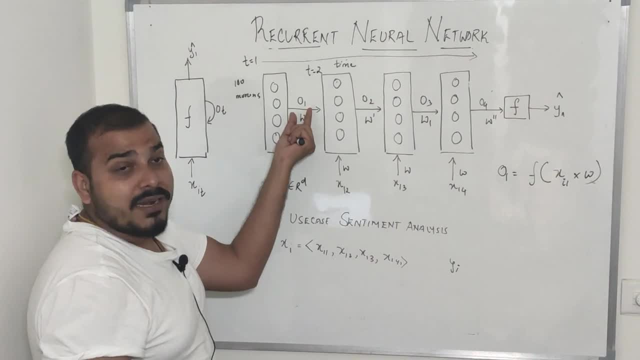 my new input will be x1, 2, but i also have one output right. this output is also going to the neuron, and when that output comes, i simply write in next to my input. i also have one output right. this output is also going to the neuron, and when that output comes, i am just going to go back and that will be myElminization to the new. sorry, over here at the front, I mean to soon number 2, so i didn't call that into the new personal information. so so you asked me what you, Audrey, had say, after which I told so In my video. they didn't call it. 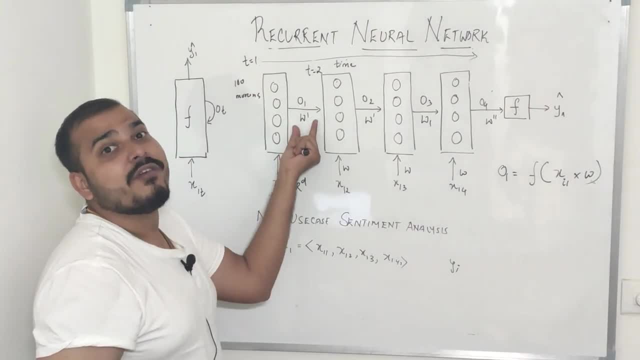 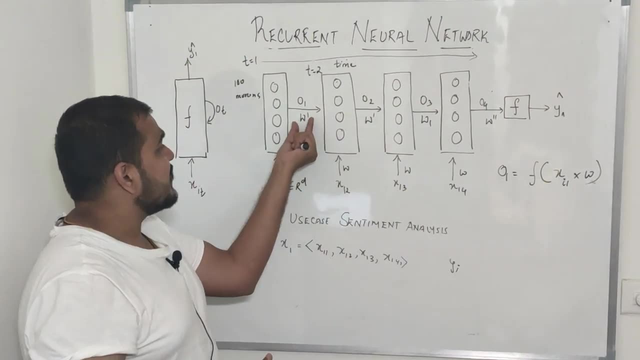 run, and when i'm passing this output, i'll assign some different weight. okay, and they have a lot of weight initialization techniques, guys, which i have already discussed in my artificial neural network. so this is my w dash, which will get initialized for this particular output. now how will my function? 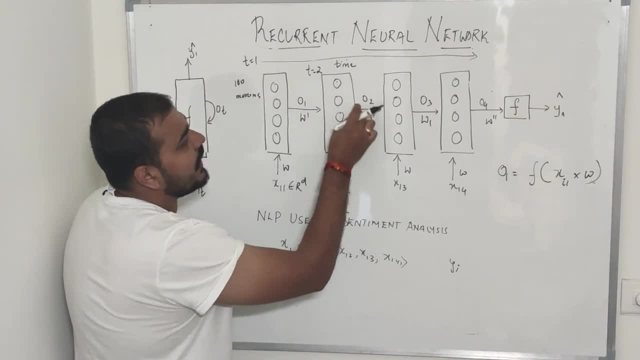 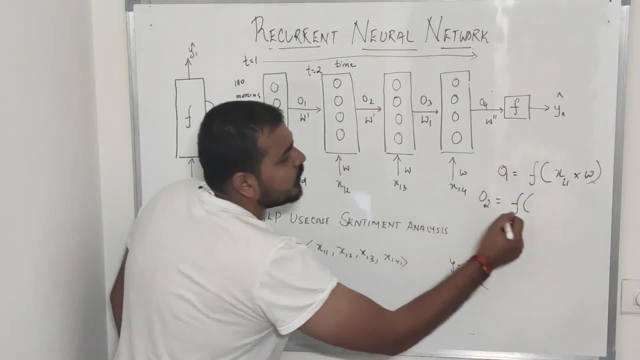 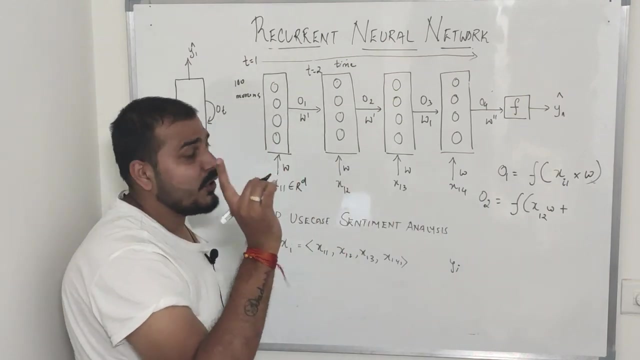 look when i'm using this data and this data and i'm getting the output o2. now my o2 will be nothing but function. first of all, i'll multiply x12 into w, so this will be my x12 into w plus. see, i'm doing. 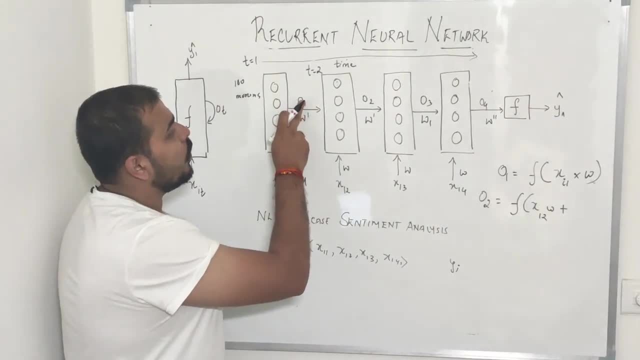 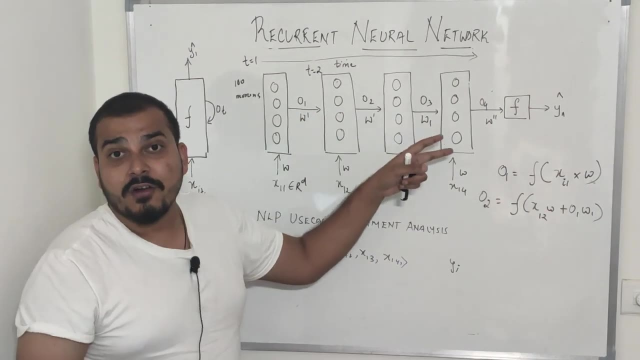 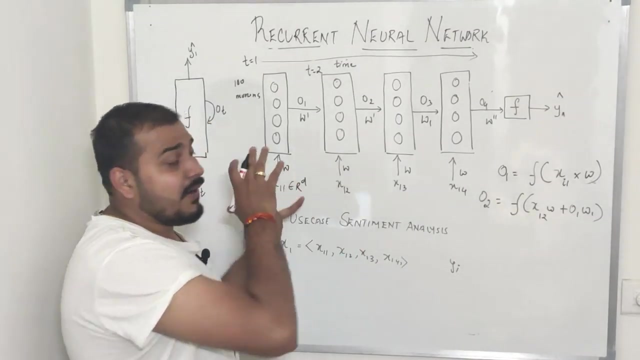 the addition operation for this one also. now, right, so o1 multiplied by w1- and this is very, very important, guys, because this is what happens in the forward propagation, in the backward propagation, again, the derivative of all this will get calculated. so that is how you know and remember. 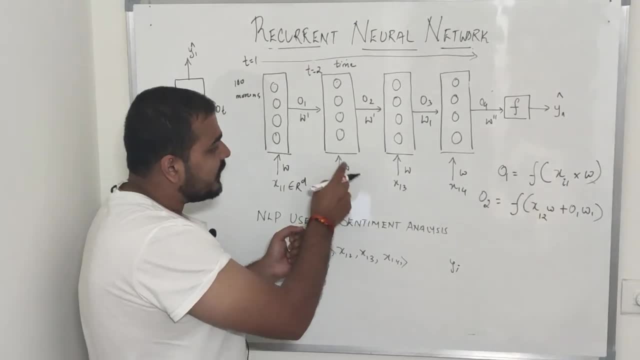 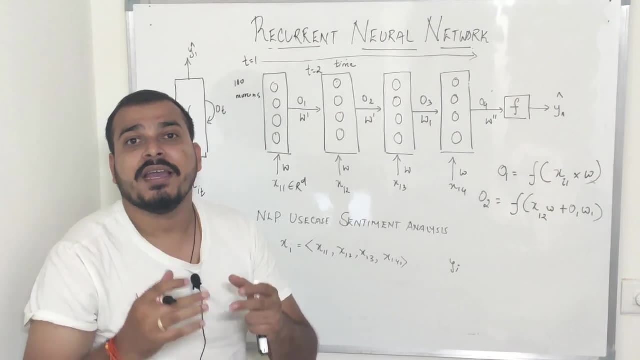 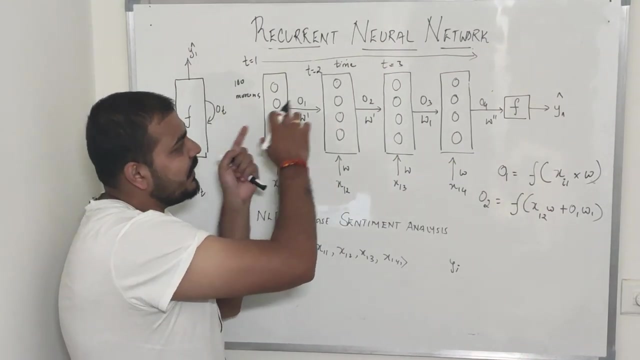 over here you. O2 is completely dependent on this, X12 and O1 and that is how sequence is actually kept. The sequence information is actually kept Now at time is equal to 3, that is, T is equal to 3 again. now this particular output will go back to the same hidden neuron, So O2 is going back over here. 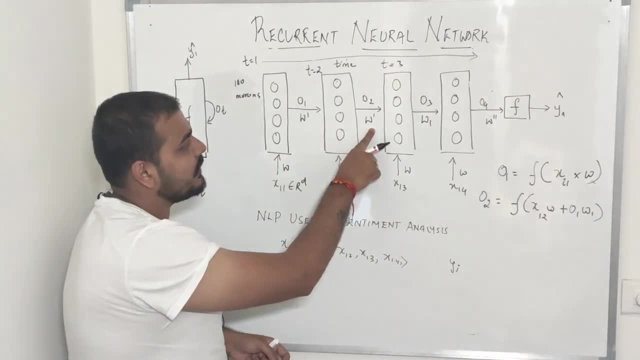 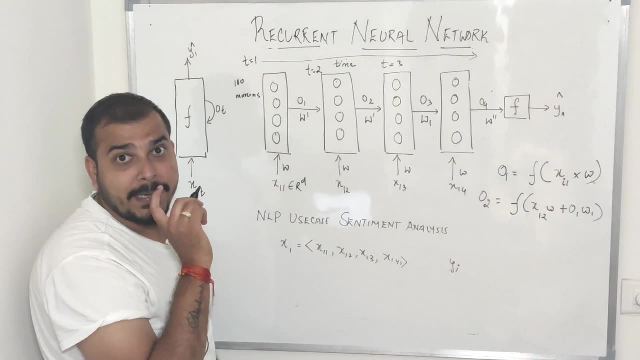 again, this weight will get initialized over here. okay, W dash, and it will be same. okay, and in this case, in the third time, T is equal to 3. X13 is getting passed right Now. in when X13 is getting passed again, this will be the same weights over here, and this will continue till the end of the 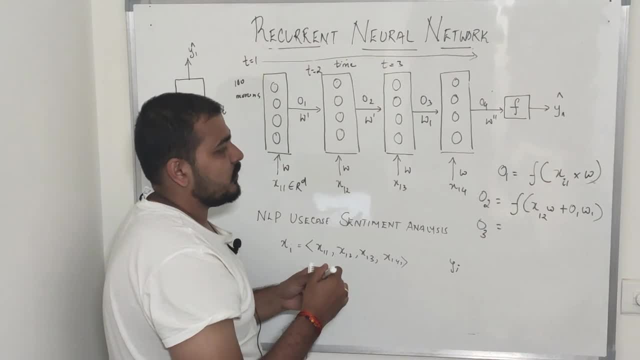 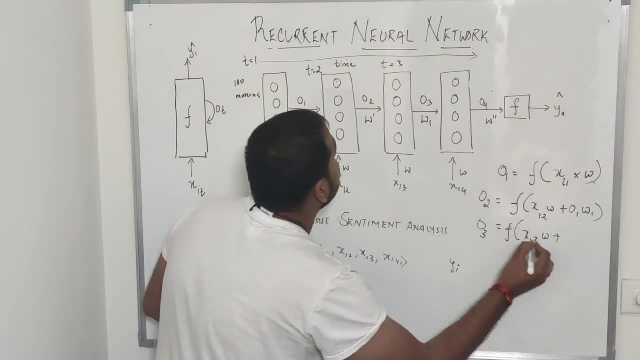 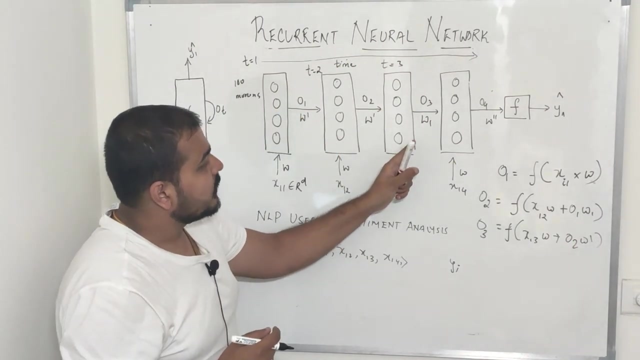 statement. So my O3- again, I can write it as my O3 will nothing be but function of X13 W plus O2 into W dash. okay, So this is my W dash and this is my O3.. Now, similarly, we can write it as O2 into W dash. So this is my W dash and this is my O3.. Now, similarly, 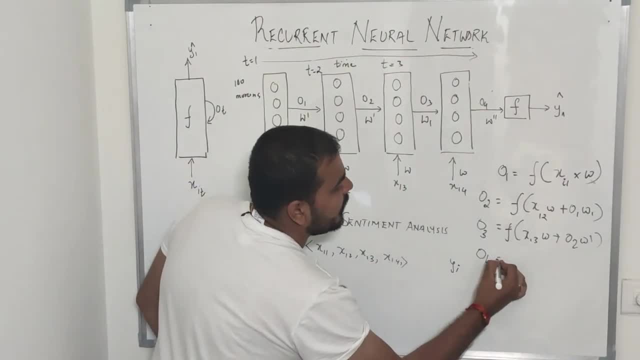 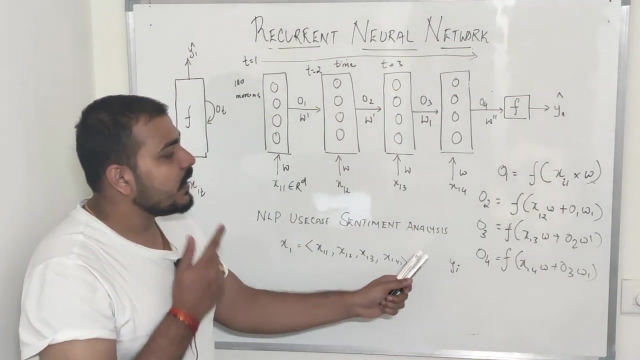 finally, my O4, which is this output will be nothing but function of X14 multiplied by W plus O3, into W1, and this is where you are getting all your output: 1 output, 2 output, 3 output, 4 in the forward propagation. This is how the function is getting computed and, guys, it will. 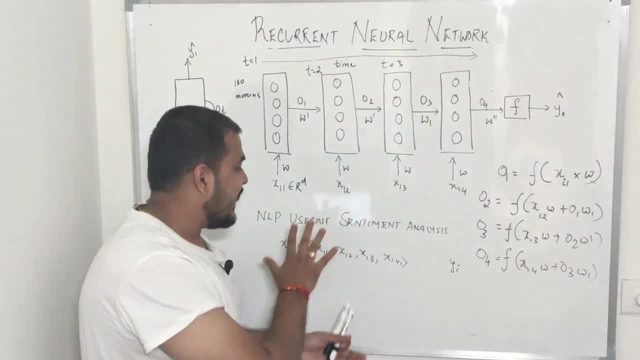 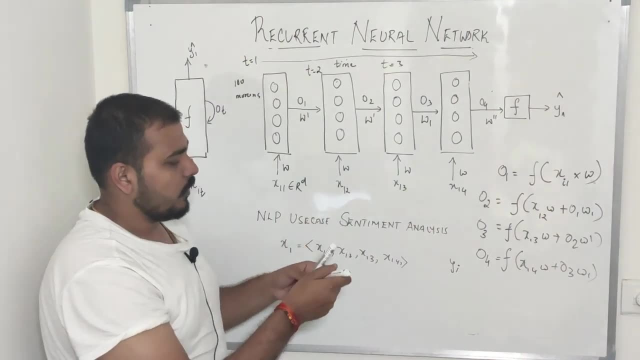 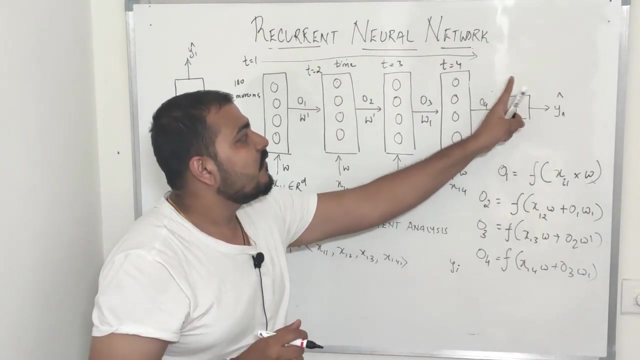 just stop in this fourth cycle, right, T is equal to 4 and sentences may have any lengths, right? So for the first sentence that you see over here, it will go till: T is equal to 4.. Now you can see over here: T is equal to 4, right Now. after you get this output function, then finally, we pass through this. 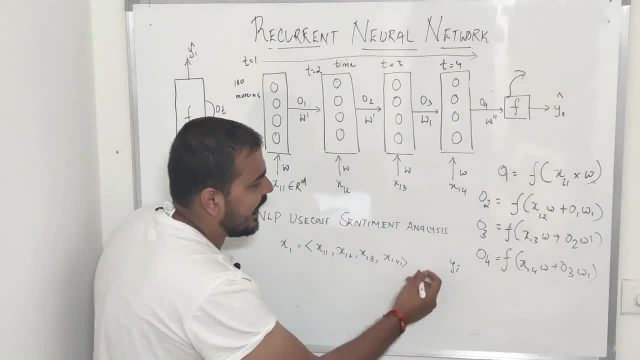 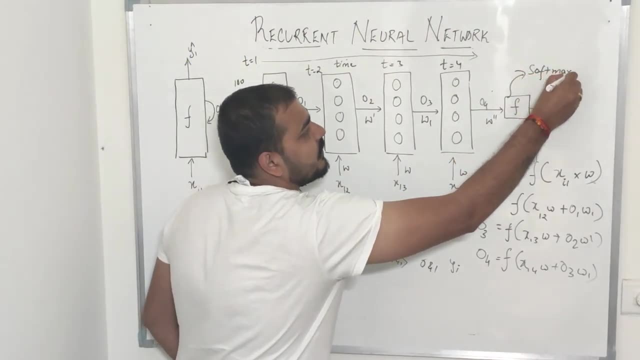 sigmoid, because, since this is an suppose, this sentiment analysis is having an output as 0 and 1. So I have to use a softmax right over here. So this will be my softmax activation function and when I am doing this and another weight will get assigned to this like W double dash. okay, 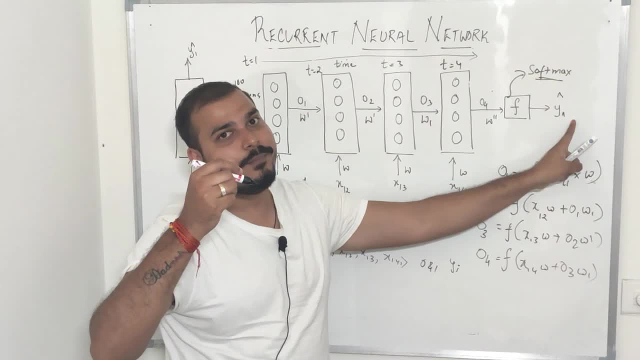 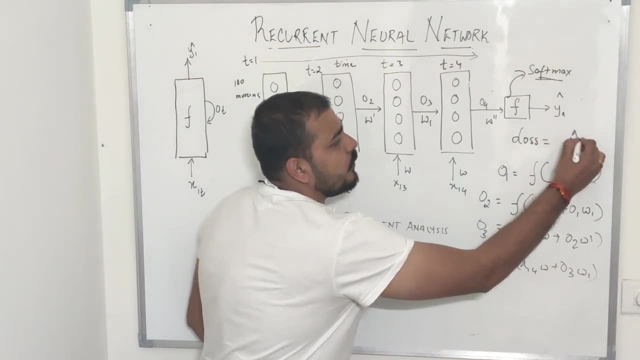 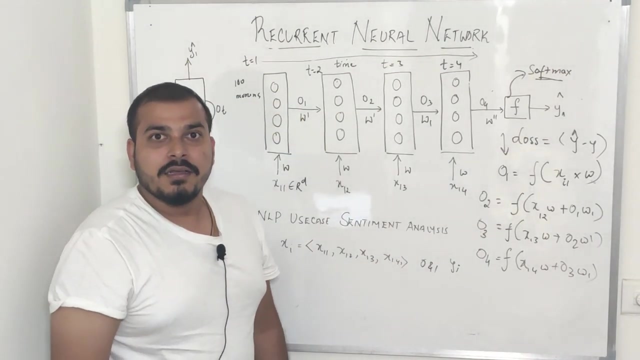 And then this will classify and this will give us our Y hat predicted value. So this is my Y hat predicted value and then I go and compute my loss function, where I will try to subtract this two value, and our main aim is to reduce this particular value. Now, once I have done this in the backward, 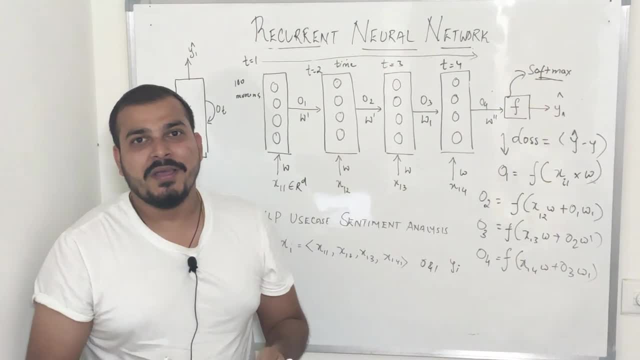 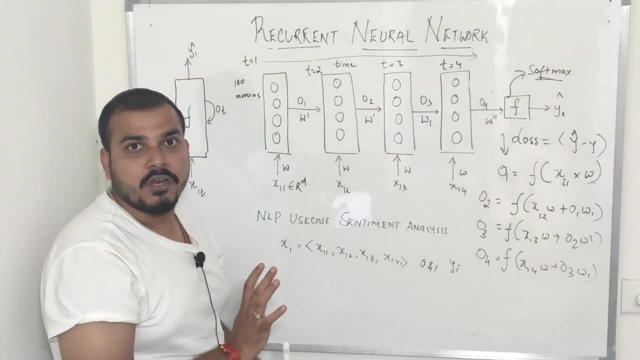 propagation. what will happen? that will be discussed in the next video. But just understand that how the forward propagation has happened, We have started from here. we have gone till the end. You know, just with respect to one statement. each and every word is can be represented into vectors. 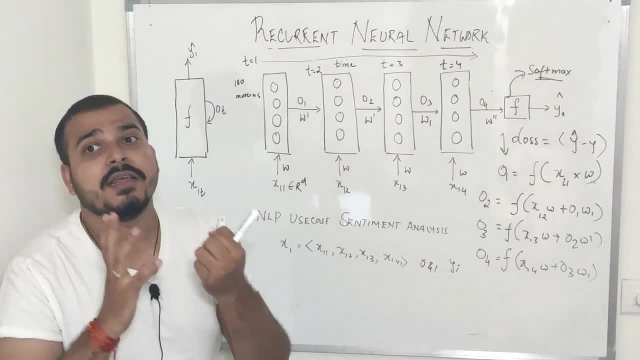 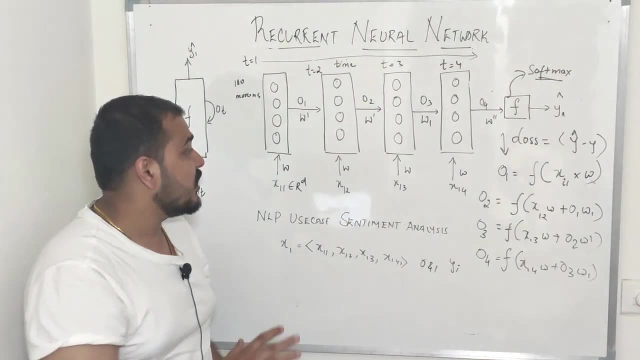 of some d dimensions and that depends on the type of vocabulary, the number of words that are present in that vocabulary. So it is very, very important how you can actually implement that. But in forward propagation this is how it goes. This main output basically means that unless and until the 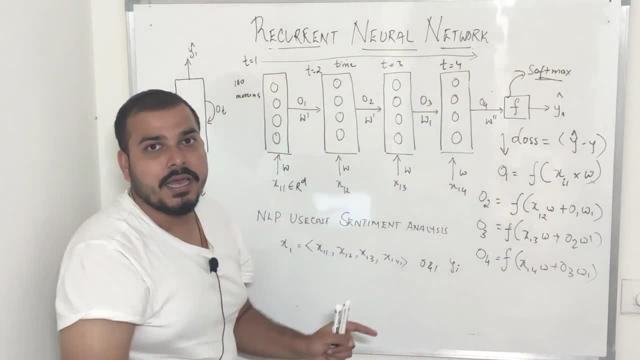 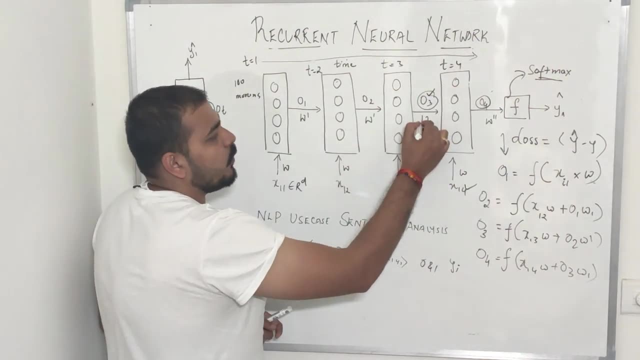 statement does not get over, this will be getting passed to the same hidden layer And always remember guys over here. the output 4 will be dependent on x1- 4. And output 3.. Output 3 will be dependent on x1- 3 and output 2.. Output 2 will be dependent on this. 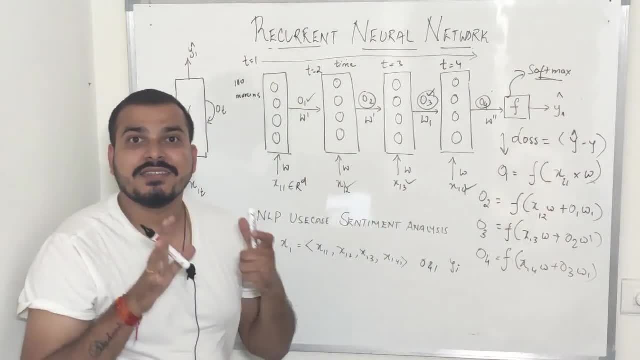 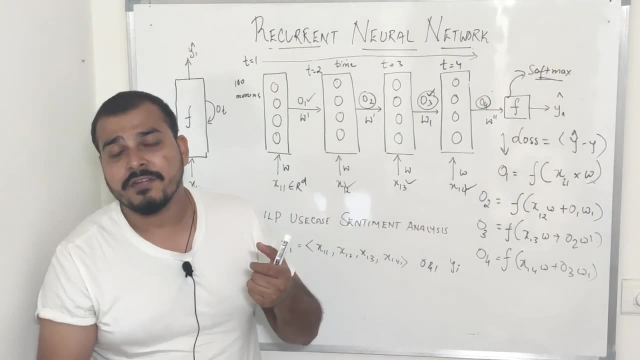 and this value. So by this the sequence information is always maintained. You know, it is not discarded, which was the problem in some of the techniques that we had like in bag of words- tf, idf, in other techniques. But in this technique the sequence information is not removed. So this is basically. 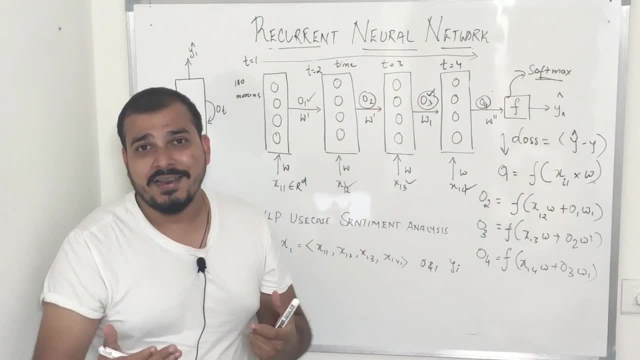 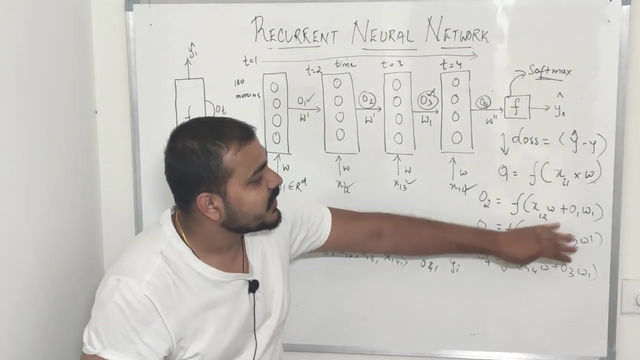 being used in many, many important applications where you know the output from that particular input and the output from that. Google assistance is very, very important, based on our statement that we usually speak, You know, and this function that we have derived over here. this is very, very important again, guys, Because in the back propagation we will try to find out the 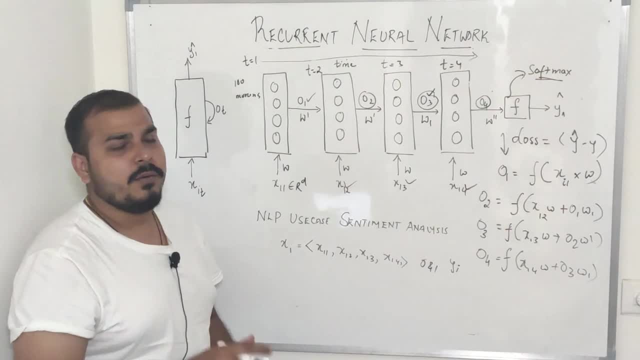 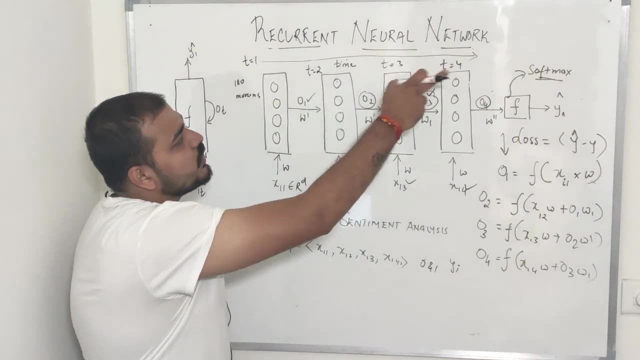 derivatives of this Right. So I hope you understood this particular video. One more change now I have to do is that guys always remember for each and every hidden neurons. when time is equal to 2, 3 and 4, you can see that one output is going. So, in order to change,